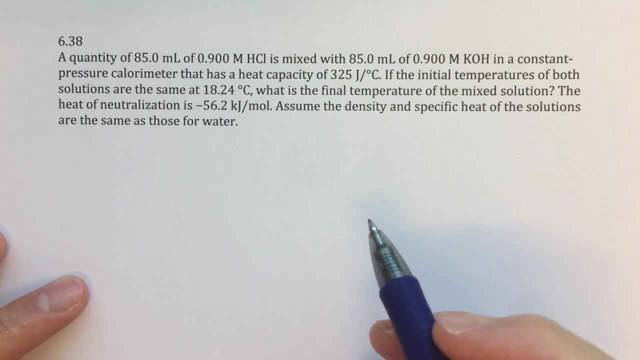 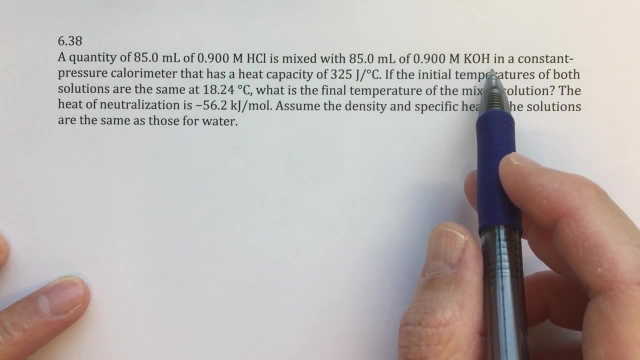 The first thing that I'm going to do is I'm going to try to organize the information that's given. So 85 milliliters of 0.9 molar HCl is mixed with 85 milliliters of 0.9 molar KOH. 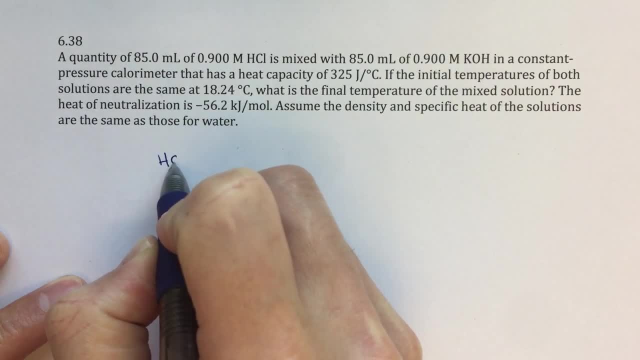 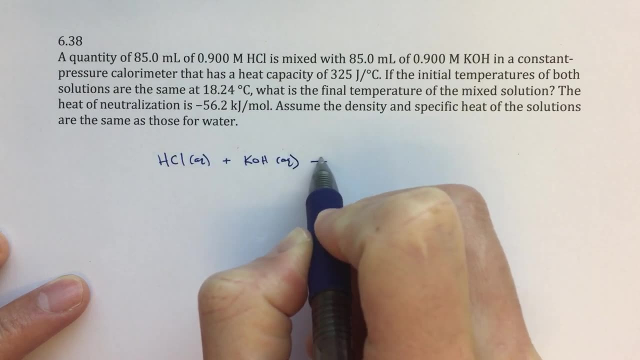 So the first thing I want to do is I want to think about the chemical reaction that's going to be occurring here. HCl- we're going to assume that that's aqueous- plus KOH- Again, aqueous goes to H2O. 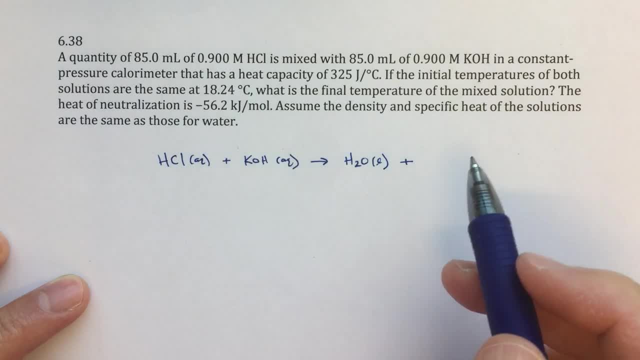 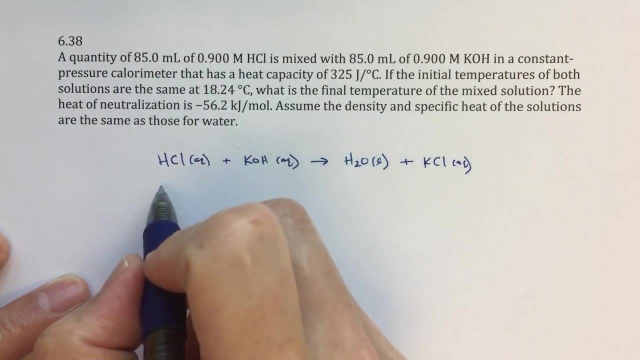 This is going to be a neutralization reaction so I can recognize a strong acid and a strong base. And then I will get KCl as another byproduct. We have 85 milliliters of each, so I will just write: 85 milliliters, 0.900 molar. 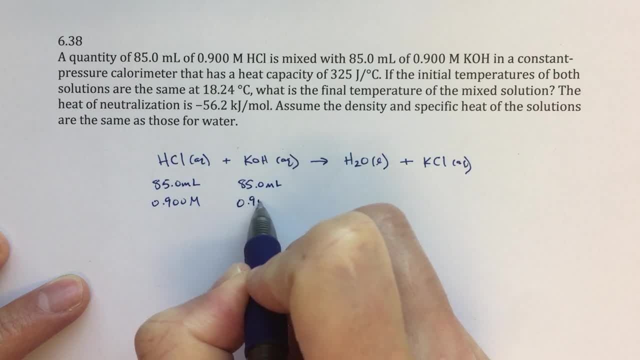 85.0 milliliters, 0.900 molar, And it might seem sort of redundant to be organizing information like this or writing this out, but it's really, really helpful, I think, as we go through the problem. 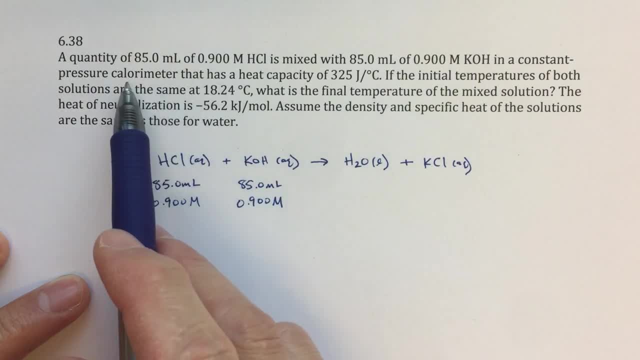 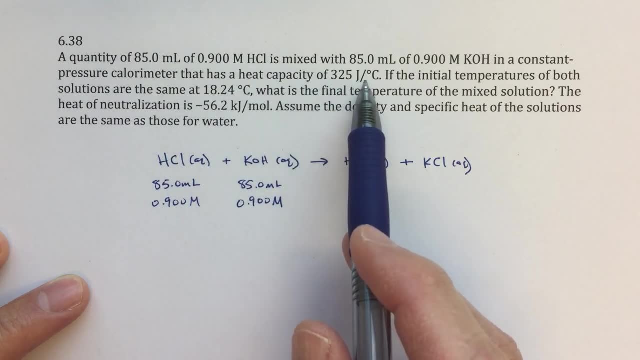 So I'd really encourage you to do that. So we're going to mix this stuff together in a constant pressure calorimeter, So we're going to be doing a calorimetry problem. There's a heat capacity of 325 joules over degrees Celsius. 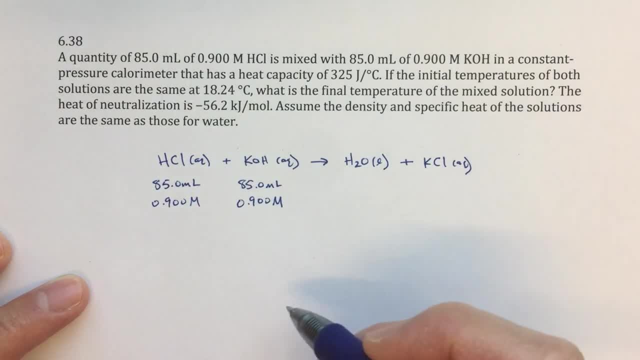 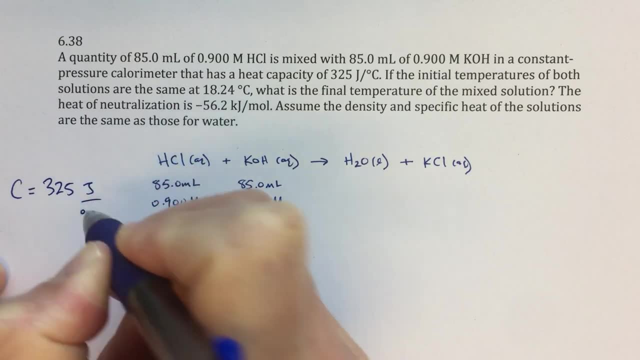 So that is what we consider to be a C value. So maybe over here to the side I'll write C. C equals 325 joules over degrees Celsius. just to organize that If the initial temperature of both solutions are the same. 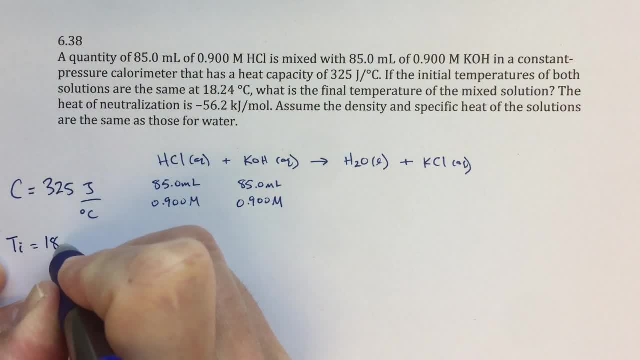 so that's going to be my T initial equals 18.24 degrees Celsius. What is the final temperature of the mixed solution? So what we're looking for is T final. So I'm going to sort of highlight that That is what my goal is for this problem. 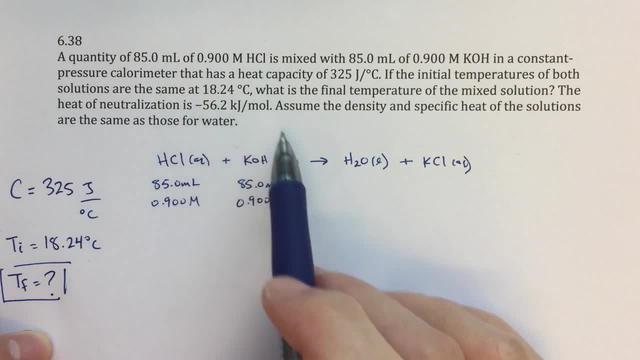 The heat of neutralization is minus 56.2 kilojoules. That's for this reaction. So that is the delta H for this reaction, minus 56.2 kilojoules. And then assume the density and specific heat of the solutions are the same as those for water. 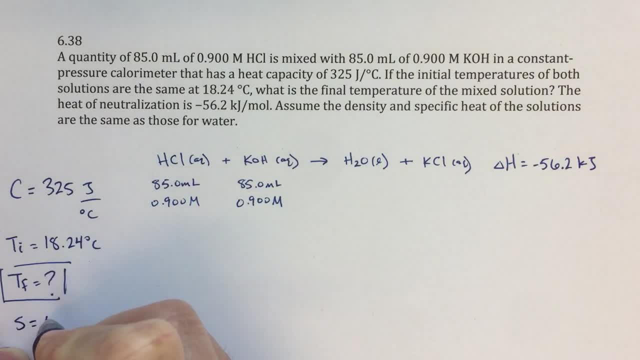 So specific heat for water- that's going to be S, equals 4.184 joules over grams times degrees Celsius, And then my density is going to equal 1 gram per milliliter. So that is all the oh. you can't see that? 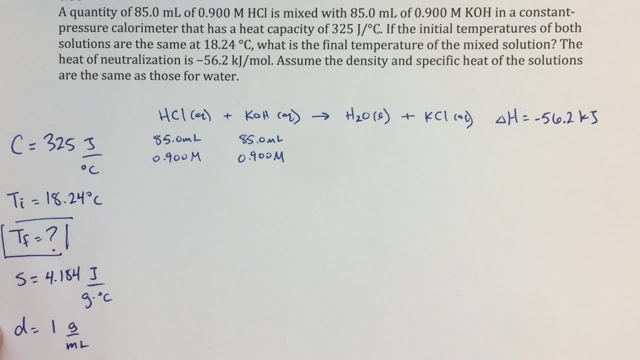 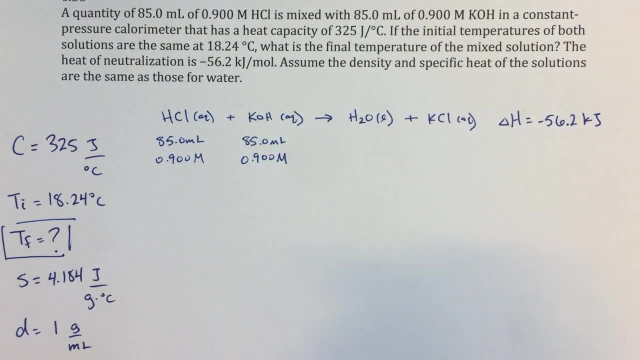 Density, but scoot that up. So that is all the information from the problem. So I spent the first two minutes just organizing the information, getting ready to do the problem, not even worrying about actually doing any calculations or anything. So now let's do that. 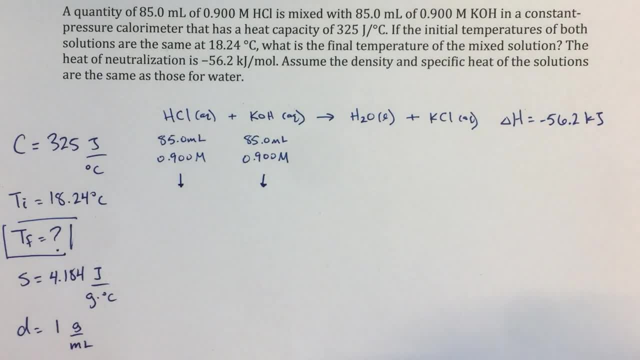 Let's worry about that. The first thing I'm going to do is I'm going to convert both of these into moles. Really, we only need to do one of them, because I can tell that they're the same essentially. So that's going to give me 0.0765 moles. 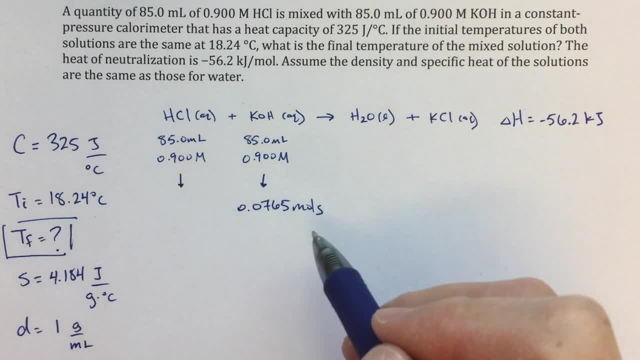 Of both. And then I'm going to use this information to figure out, well, when I do that mixing, when I mix these two things together, how much energy is going to be released. And I want to think about that because I've got that information. 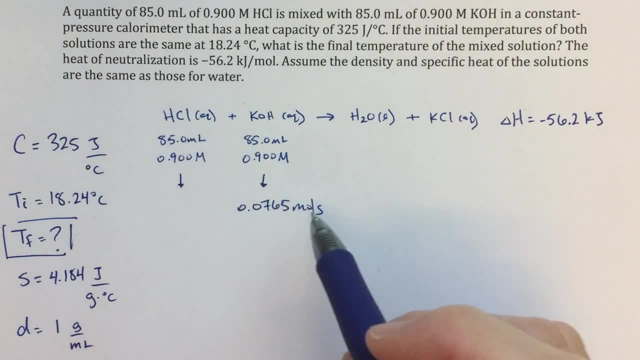 You know this. minus 56.2 kilojoules. that's per mole. So if I've got 0.0765 moles, then I'm just going to multiply that by minus 56.2 kilojoules over 1 mole. 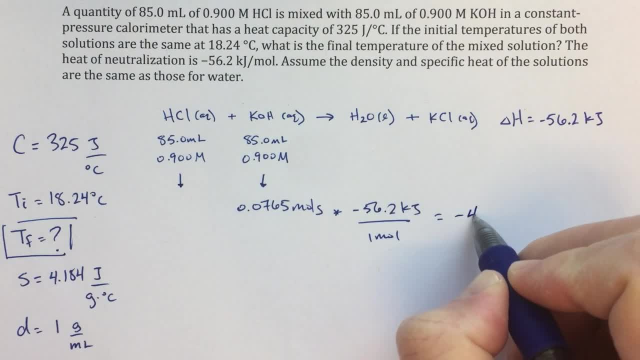 And that value is going to be minus 4.2.. Minus 4.2993 kilojoules. So what this represents, this represents the amount of energy released. So let's sort of annotate that Energy released by the chemical reaction. 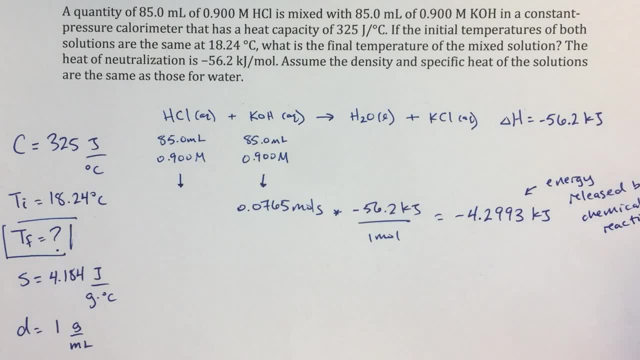 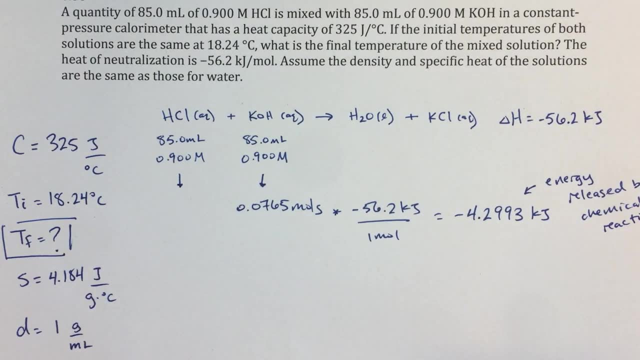 Or we might call that the system. So by the chemical reaction, When I mix these HCl and KOH solutions together, that amount of energy is going to be released, Minus 4.2993 kilojoules, And that amount of energy it's going to be then applied. 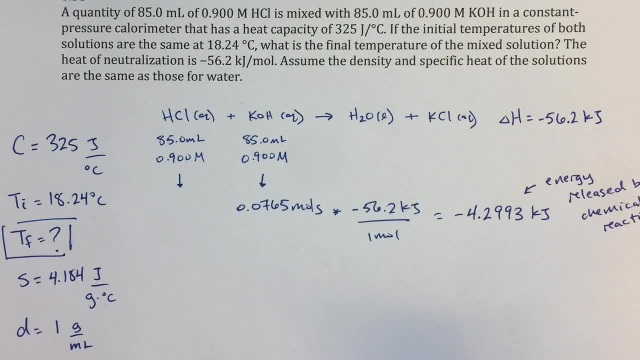 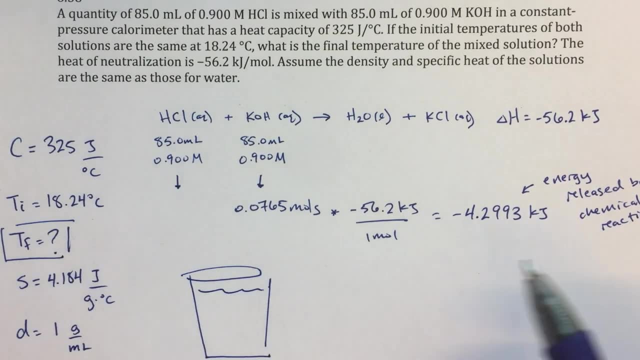 To the calorimeter and the actual water solutions that those solutions make up. So if I draw a little picture here, This is going to be my calorimeter. with my solution I'm going to have 85 plus 85 milliliters, So I'm going to have 170 milliliters total. 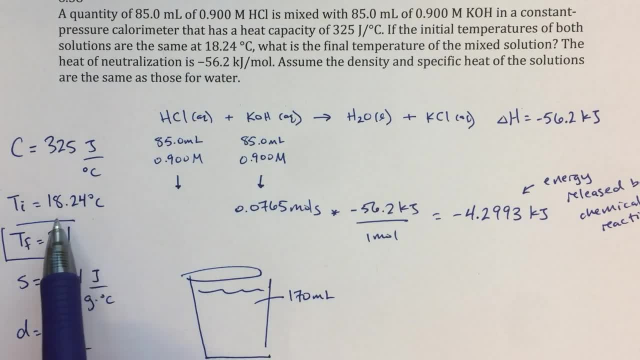 I've mixed my two solutions together in there. The initial temperature is going to be this: 18.24 degrees Celsius, The specific heat and density that's going to be for this solution That I have in my calorimeter, And then this other piece of information: 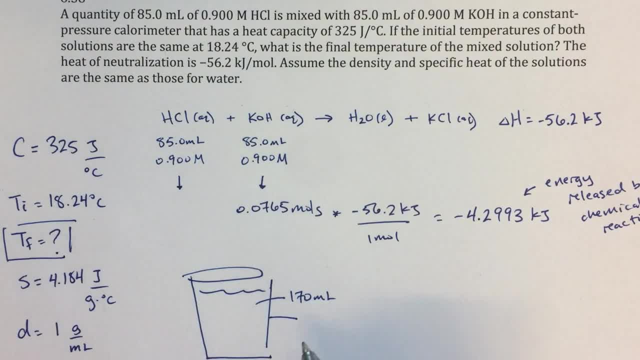 It's really telling us what the heat capacity of the walls of the calorimeter are. So we're going to say that that C equals 325 joules over degrees Celsius. So it's going to take a little bit of energy to heat up the actual walls of the calorimeter as well. 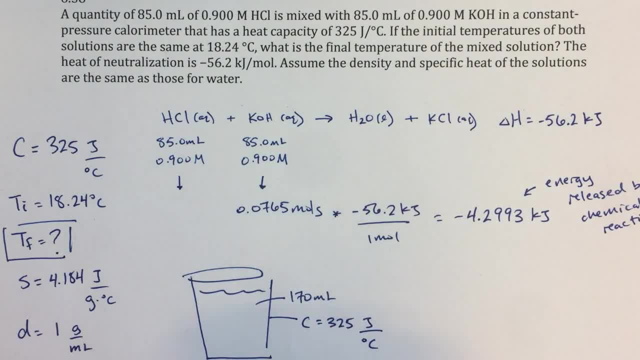 So now we're going to apply this energy to the actual calorimeter. So the way that I would do that is: first I'm going to change the sign. I'm going to say positive 4.2.. 4.2993 kilojoules is absorbed by the calorimeter. 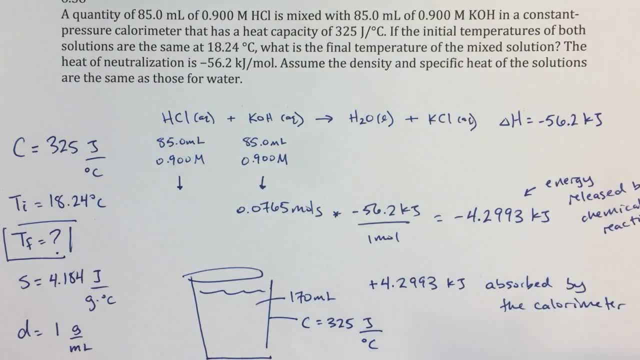 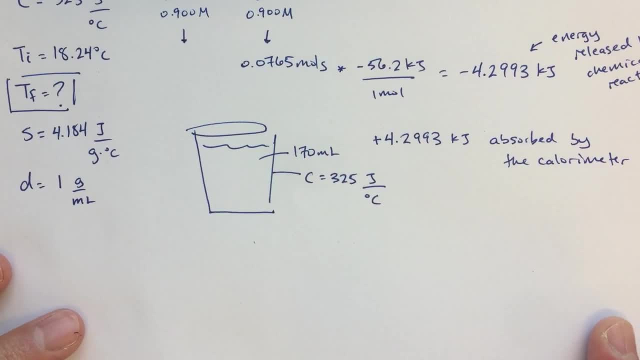 So this same amount of energy that is evolved is going to be absorbed by the calorimeter, And then we're going to apply that to change the temperature and figure out what the final temperature is going to be. So to do that, what I would do is I'm going to convert this 4.2993 into joules. 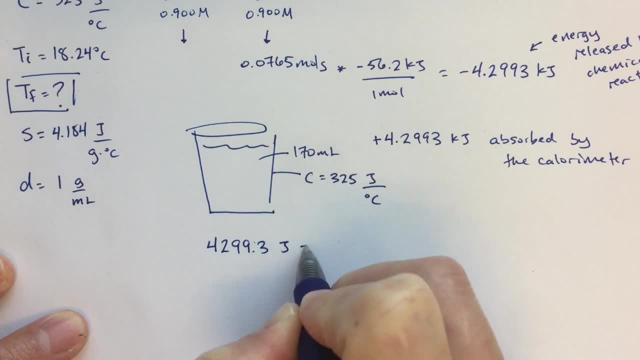 That would be 4,293.. 4,293 joules of energy And that's going to equal my water solution absorbing that energy and also the calorimeter absorbing the energy as well. So that's going to equal 4.184.. 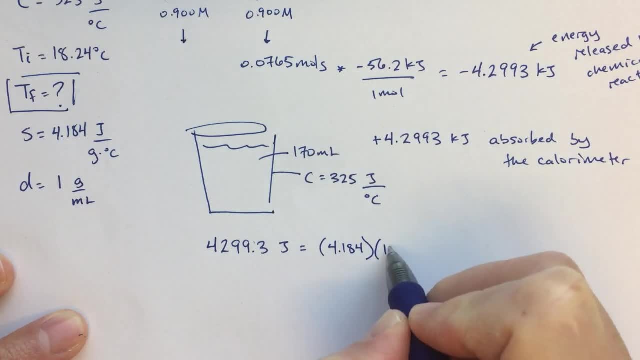 So here I'm using the Q equals SM, delta T type equation. 170 is going to be my mass, So that's going to be the mass of the water, One gram per milliliter. So 170 milliliters, 170 grams. 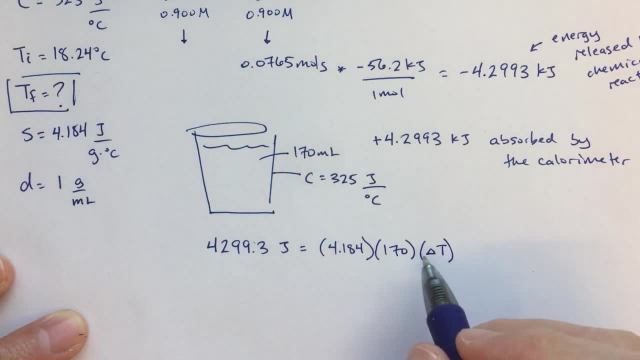 And then I'm going to put in delta T So we could do T final minus T initial, But I think for me I always just like I like doing delta T if we can. Now there's going to be another component to this equation. 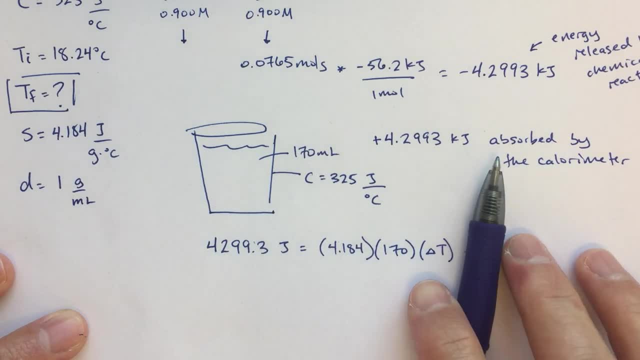 So this equation here, So let's cover this up as that plus This equation here- would be if all the energy is applied directly to the calorimeter, But in fact we are directly- to Excuse me- Directly to the water. 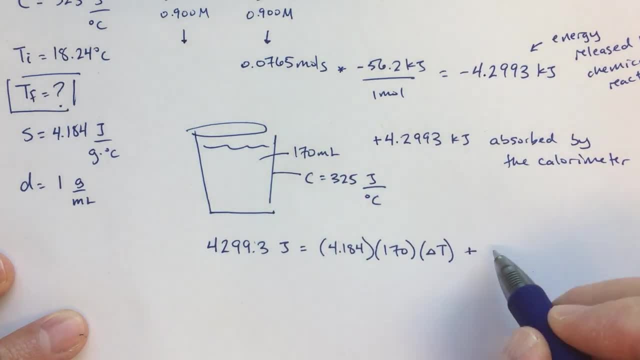 But in fact we also have to take into account this calorimeter bit. So the heat capacity for the calorimeter is 325 joules over degrees Celsius. So that's going to have to change temperature as well, And we're going to. 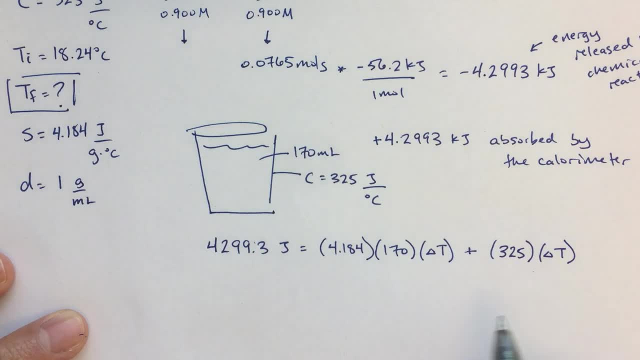 We're going to assume that that has the same initial temperature. So now I'm going to solve this equation for delta T And I get a value of 4.15.. And then to find my T final, I'm just going to add 4.15 to my T initial.